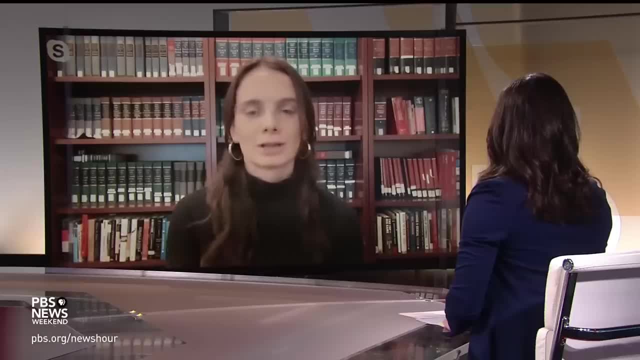 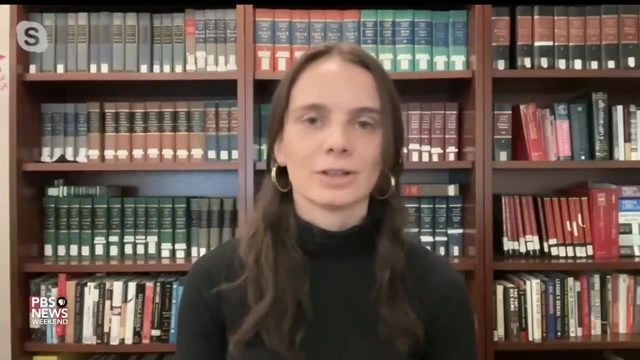 sign off on rejecting that claim and saying: we're not going to cover it. In two months last year that happened in an average of under two seconds. So these medical directors were essentially saying: for you know, 50. patients at a time, they wouldn't even open a patient file, but they were signing their name off and saying: 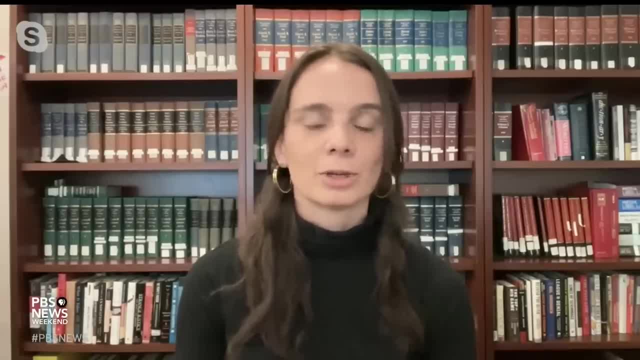 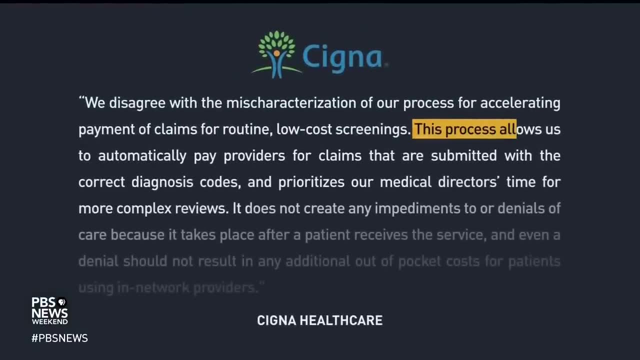 actually this claim is not medically necessary, and so we're not going to cover it. Now I want to read to you from a statement that Cigna has provided. First, they say that this automated process allows us to pay providers for claims quickly and automatically and allows medical 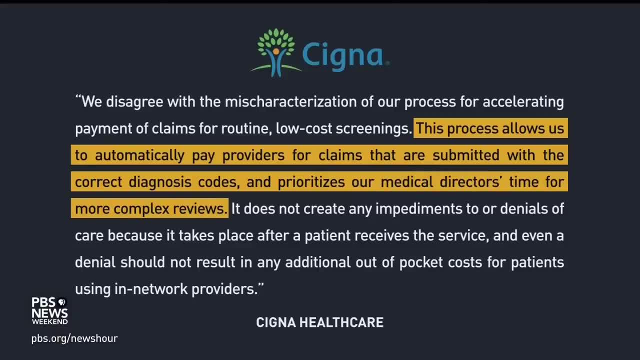 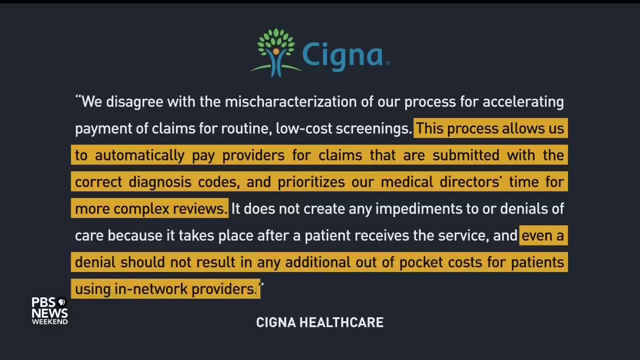 directors time to look at more complex reviews. It also says that even a denial should not result in any additional outcome. It also says that there are no out-of-pocket costs for patients who are using in-network providers. What did you find related to those two statements that Cigna makes? Yeah. so, on the first statement, it's true that some of the claims that are processed through the system which is called PXDX, if they match the diagnoses and the treatments on the list, if the code sees that there's a match there, they will be automatically approved. However, then there's a batch of them that get automatically denied. 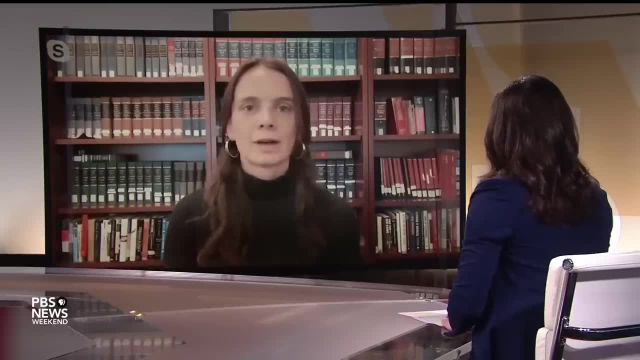 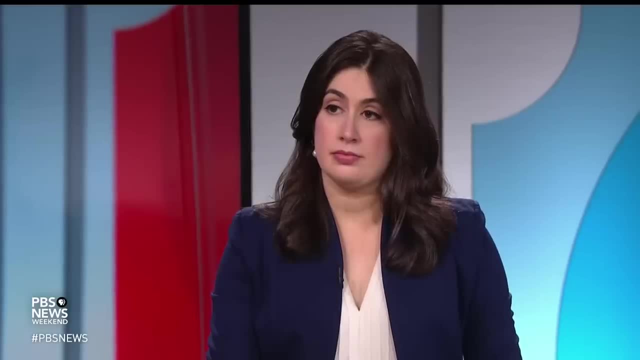 And that's really what we're focusing on on the story is the batch of claims which we found, you know, in two months last year exceeded 300,000 claims, So it's not an insignificant amount. And to the second point about you know that this shouldn't result in any out-of-pocket costs for patients. 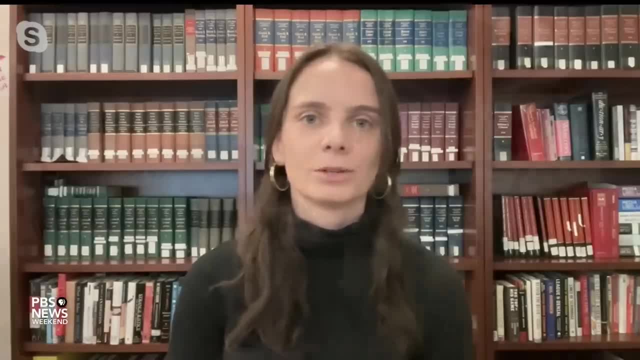 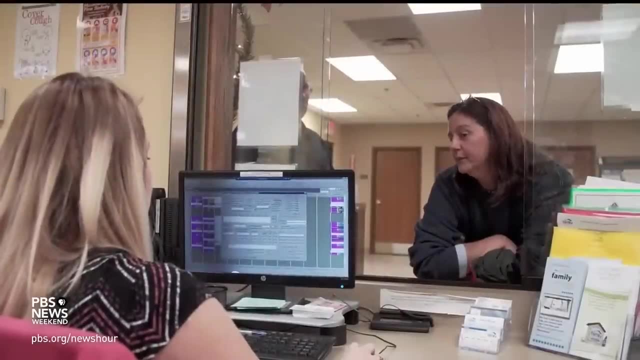 Unfortunately, the reality is is oftentimes, when we go to a doctor, a nurse or to see a health care provider, we often have to sign off on a form, And in that form we're saying that you know we'll take responsibility- financial responsibility- for them. 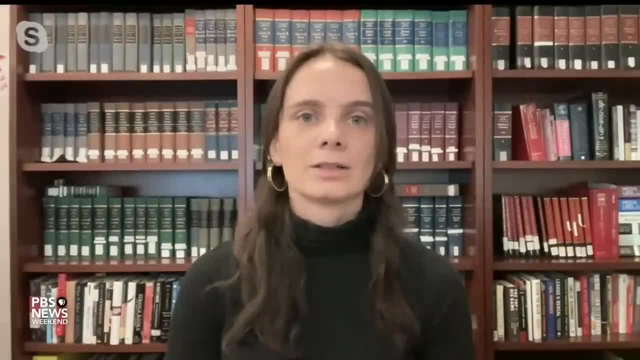 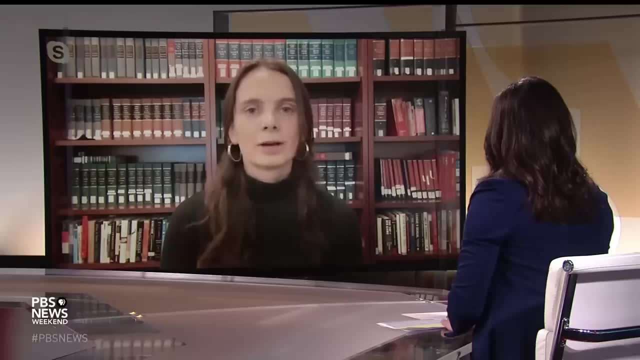 We'll take responsibility for this outcome of this care, And so it does often get shunted onto the patient. And what kind of procedures are we talking about that are getting routinely denied? Yeah, So, unfortunately, we were trying to look for a comprehensive list of all of these claims that process through the system. 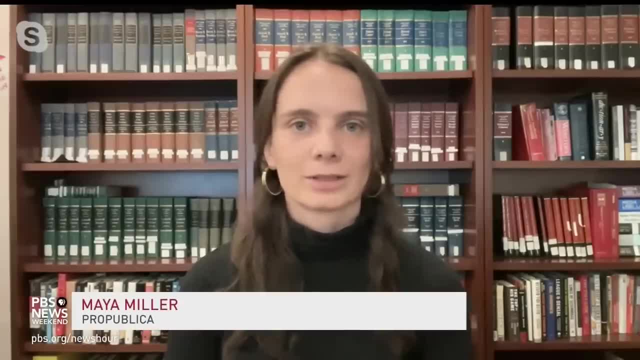 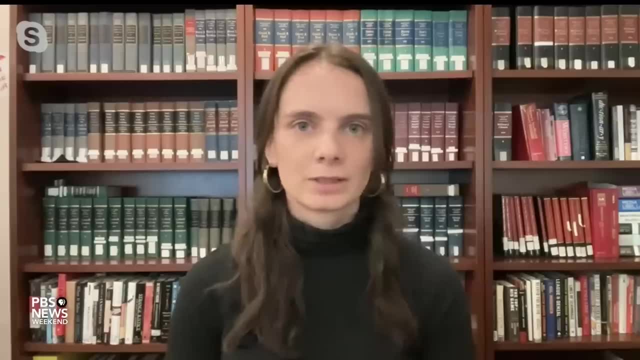 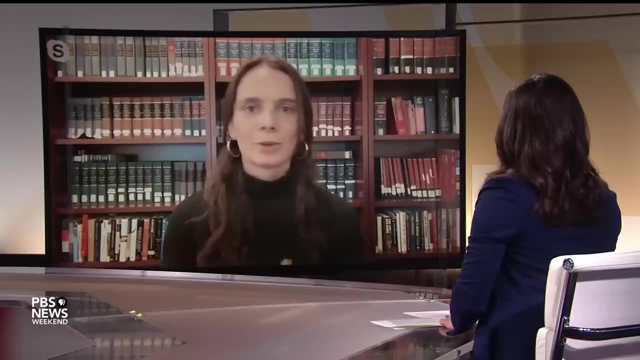 We know that not all of the claims that Cigna has end up going through the system, But of those that do. we learned that vitamin D testing is labeled as part of the system. We learned that autonomic nervous system testing to test, like whether your nerve, your nerves, are working well. If, oftentimes, if you have diabetes or other autoimmune disease, you can have some nerve damage in your fingers or your toes, And so testing to kind of figure that out among other conditions. Unfortunately, we could not find a comprehensive list of all of the different procedures that are tagged for the system. But those were two that we were able to conclude from our reporting. Cigna and all insurers, frankly, in claims denial issues will say, well, there's always the appeal process. What does that look like in reality? Yeah, So one in seven claims are denied across the country and health insurance claims So it affects a lot of people. And yet one study found that point one, point one percent of all people who experienced those denials actually took it to a step to do a formal appeal One year. And so we're in a state of emergency where we're in a state of emergency, where we're going about your day to day. 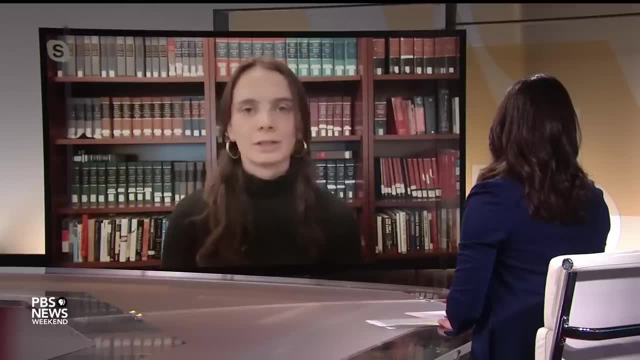 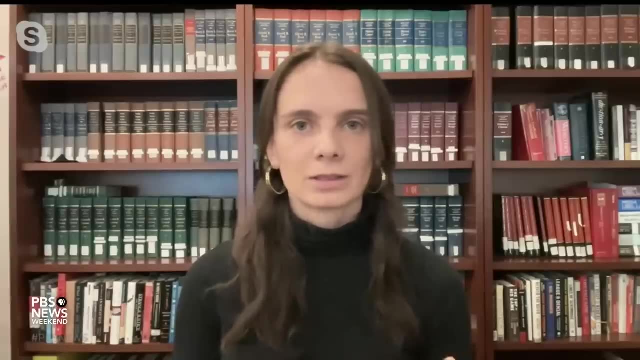 Maybe you're facing an illness or you're facing a disease, a chronic disease. It's hard to find the time and wherewithal to be able to figure out how to appeal these claims, And the reality is that very few people do. And you know we actually found through our reporting that Cigna had a presentation in which they were putting forward the idea to put autonomic nervous system testing through the system And in the cost benefit analysis assessing whether to do this. They assumed that they would. they assumed only 5% of patients would end up appealing this, And that was part of the calculation of whether to put this test into this process or program or to leave it out. Now, Cigna is not the only insurer with some kind of automated system exactly like this. 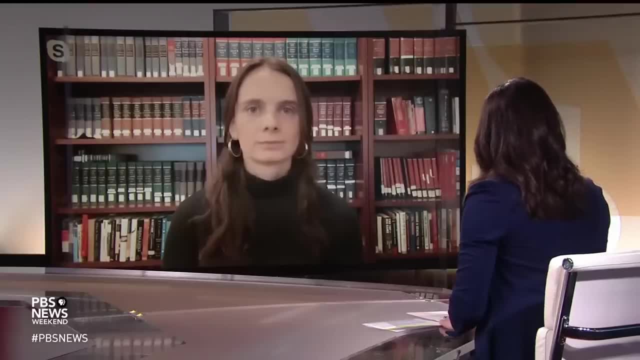 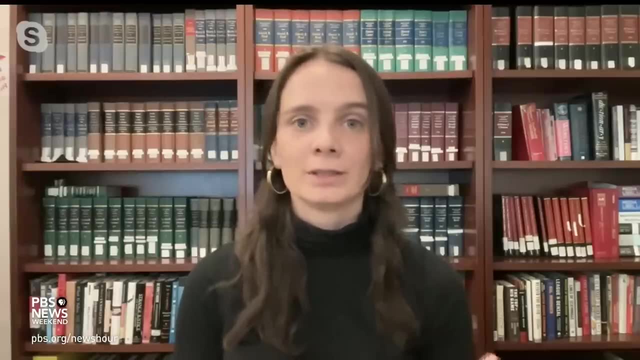 Do you have a sense of how prevalent automated systems are right now in the health system at large? It appears to be pretty prevalent And you know, insurance companies are dealing with millions and millions of claims, And so, in order to stay on top of those and to maintain efficiency, which is what they've said- 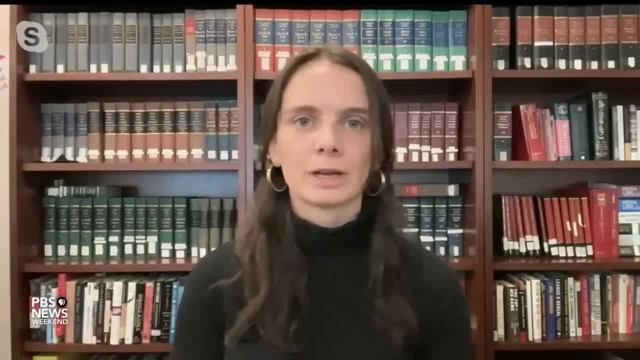 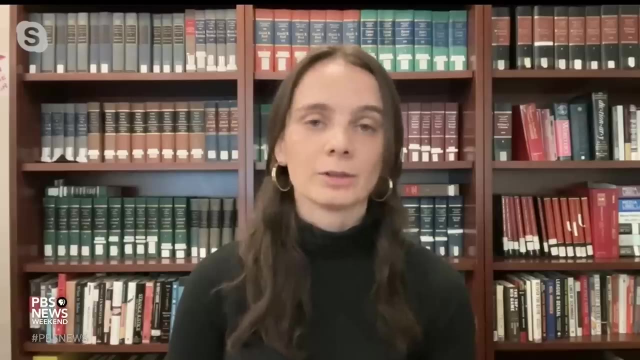 they've, you know, turned to these algorithms and computer coding programs to be able to process claims as quickly and efficiently as possible, is what they say. So it seems that this kind of technology is pretty prevalent across the industry, although we're still reporting that out for other insurance plans and trying to confirm that. 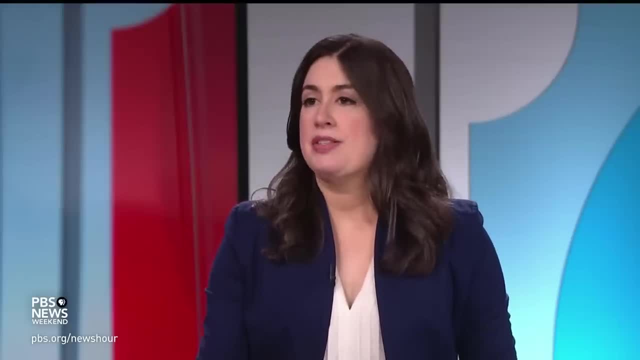 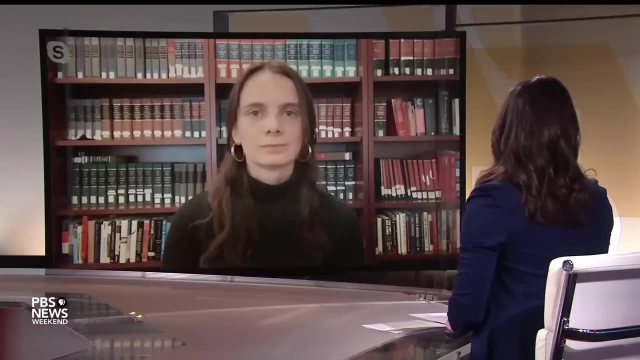 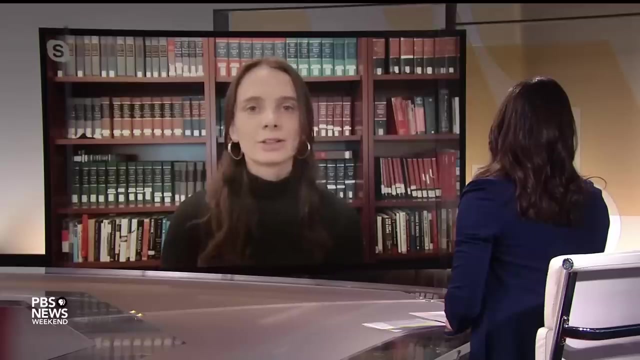 But, yeah, it seems like it's pretty pervasive. Lastly, Maya, there was a robust debate happening about the hazards of using AI. Where does this conversation fit into the broader debate about the utility and the hazards of using artificial intelligence? Yeah, that's a great question and one that we're actually, you know, posing to regulators right now. 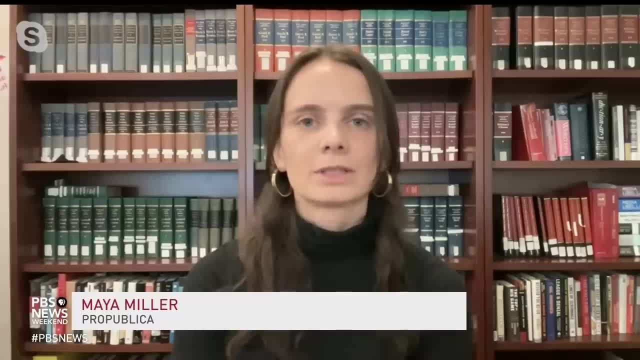 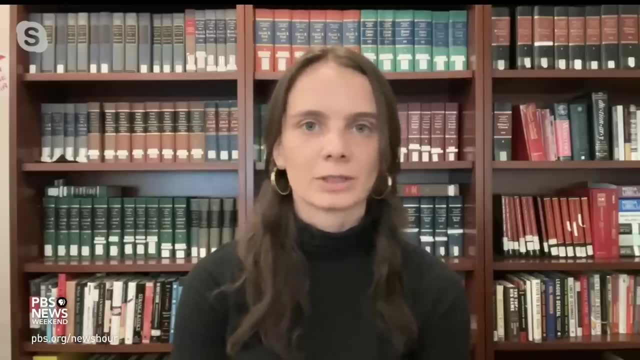 The former insurance commissioner of California, Dave Jones, was telling us that you know, in the statutes you need to have a thorough, fair and objective assessment of these patient claims. And he was saying that if an insurer, if a medical director or a company doctor for an insurance plan is really looking at a claim in less than two seconds, 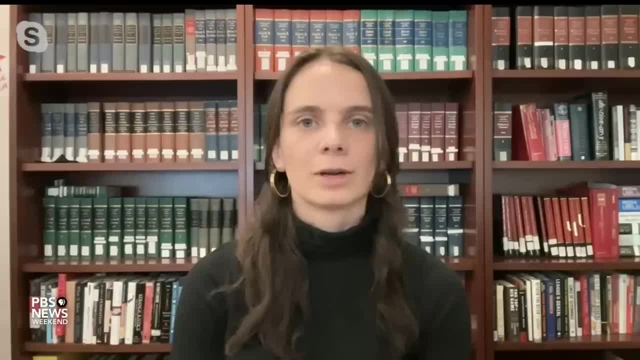 in an average of less than two seconds. can you achieve that result? So yeah, I'd pose that question really to the lawmakers, regulators, and to see you know where they would stand on that. Maya Miller, with ProPublica. thank you so much for your time. 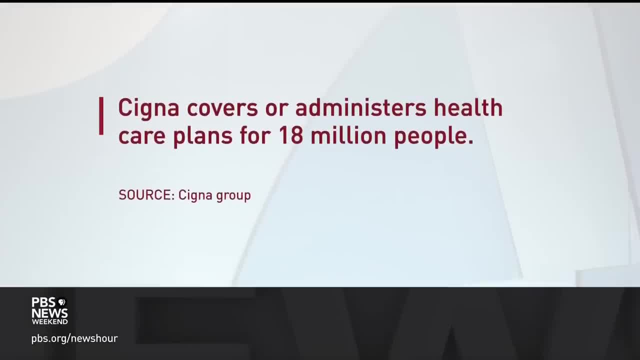 Thanks for having me. Thank you.